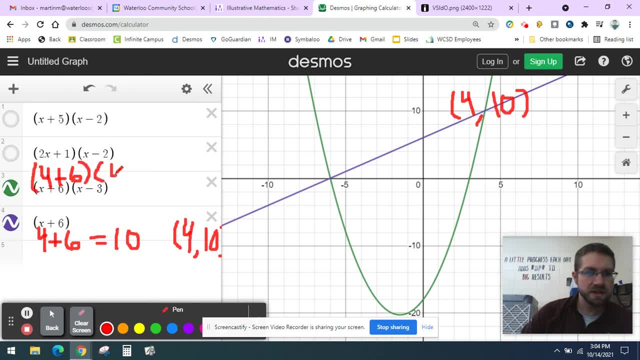 the x, I'd have four plus six in the first parenthesis and four minus three in the second parenthesis, And if we simplify that I would be 10 times one, Which you guessed. it is still 10, which tells me that four comma 10 is also a point. on the second: 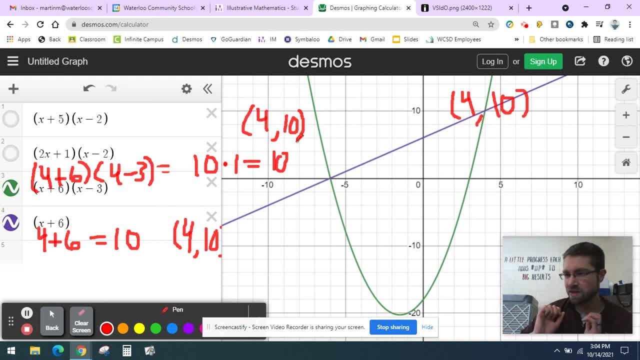 function. So for the same value of x, they have the same output, the same y value. And this would also work with the point negative six zero. I'm not going to do that for time's sake, but let's just that's what you're finding when you find the intersection points. Finding the intersections is 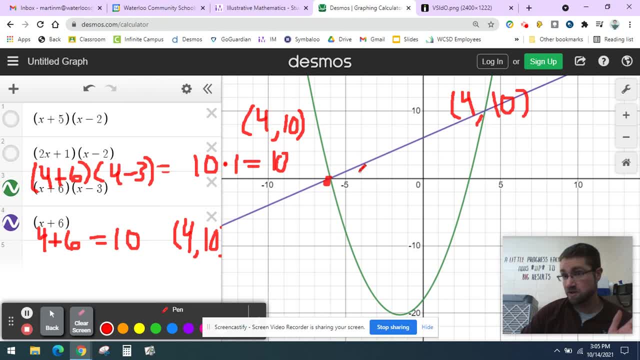 also sometimes called solving the system of equations. So that's what you're finding when you find the intersections. Oh, okay, Now, more importantly, I want to show you how to do that with algebra, because that's a skill that we want you to have. So here's what I'm going to do. I'm 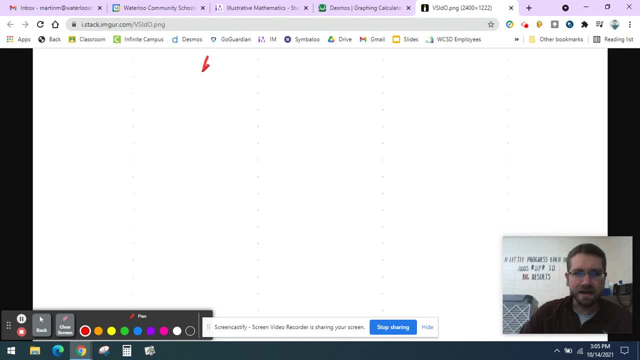 going to think to myself: all right, well, I've got these two functions, I'm going to write them out here: x plus six times x minus three, And I want to know where does it intersect with just x plus six? That was the other function, all by itself. 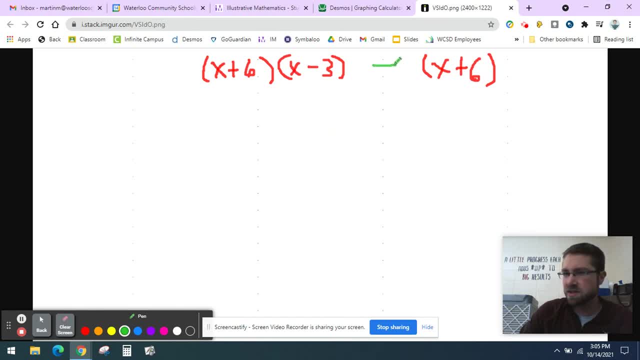 Now, if I want to know where they intersect, I'm essentially thinking to myself: where are they equal to each other? Okay, So I'm setting them equal to each other And then, if I solve this, if I get x by itself, I will be finding the x coordinates for the intersection. 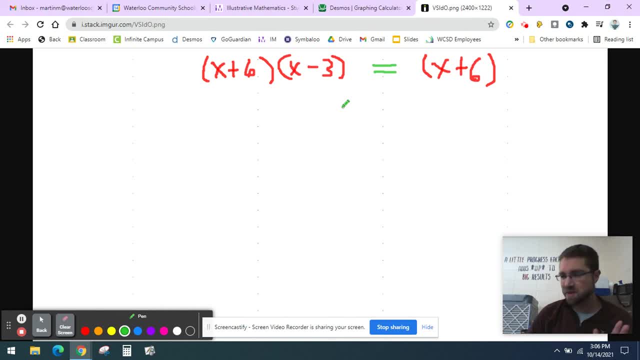 points, And I already know what they're going to be because we just saw them on the graph. But let's suspend our disbelief for a minute and say we're starting from scratch, Okay. So how do I solve this? How do I get the x values algebraically? Well, I'm going to do a little. 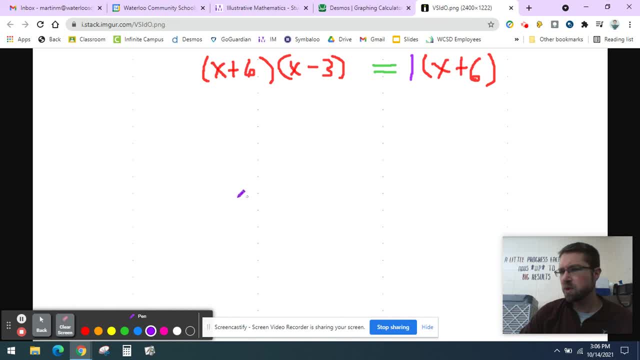 thing here. that's going to seem kind of weird at first, but I'm going to put a one in front of the x plus six, because there's one of them And because these problems are a little bit of a setup that's going to help us out a lot later on. Okay, Just take my word for it. Multiplying by one: 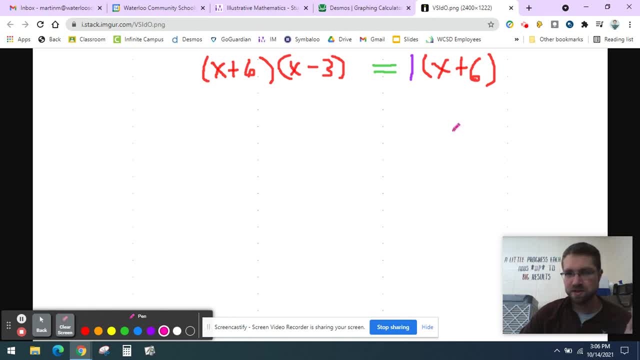 doesn't change anything, So it's not hurting anything to put a one out in front. Now, here's what I'm going to do. I know that if I put a one in front of the x plus six, I'm going to get a one. 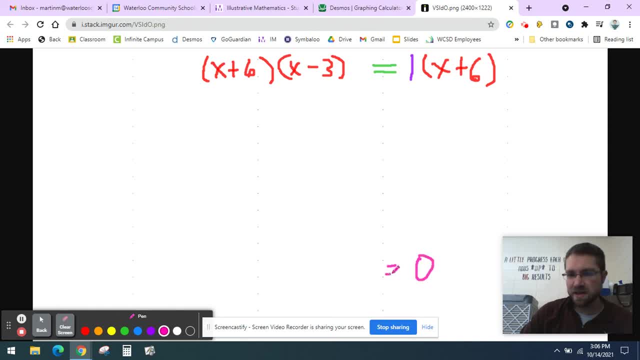 at the end of the day, I want to end up with something like this: I want two factors, or I guess it could be more than two, but it's going to be two. Two factors multiplied together, equal to zero, Because if I have that, then I can use the zero product property and that will let me. 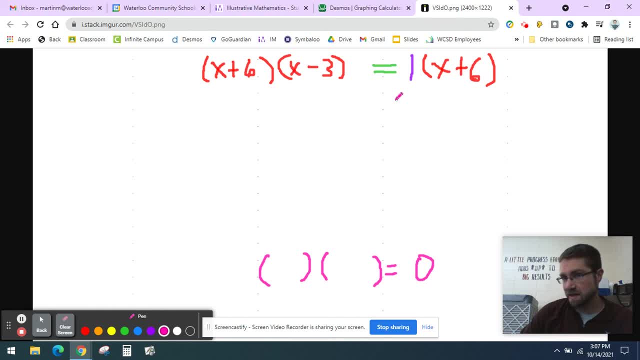 solve for x, right? That's what we've been doing a lot lately with polynomials, right? Getting the x intercepts is using the zero product property, Okay. So, anyway, how am I going to get there? Well, I need zero on one side, don't I? So I'm going to cancel out. 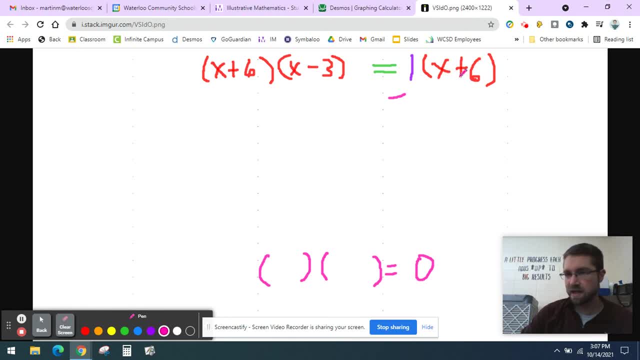 everything I have over here And to cancel out one times x plus six. I'm going to subtract away one times x plus six from that side And that would leave me with zero, But of course the equation would not be balanced. okay, It's not equal unless you do the same thing to both sides, right? 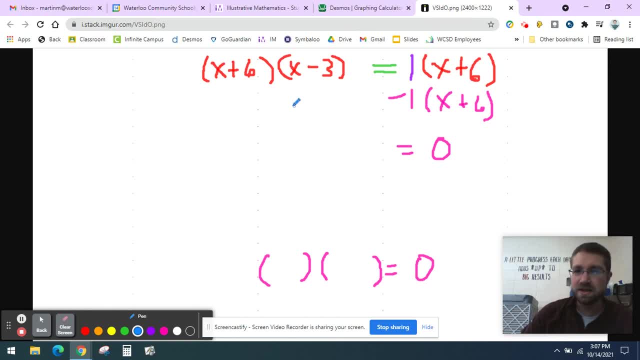 So if I subtract away one times x plus six, I'm going to subtract away one times x plus six. I'm going to subtract one times x plus six from over here. I am also going to subtract one times x plus six from this side. It would be very tempting to just cancel out those x plus sixes, but that's. 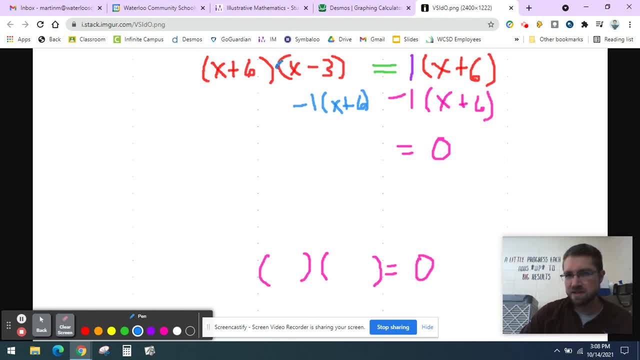 not the way this works. okay, Because right now there's technically multiplication going on right there and you can't add or subtract until all of your multiplication is done. right? That's how order of operations goes, So I can't. 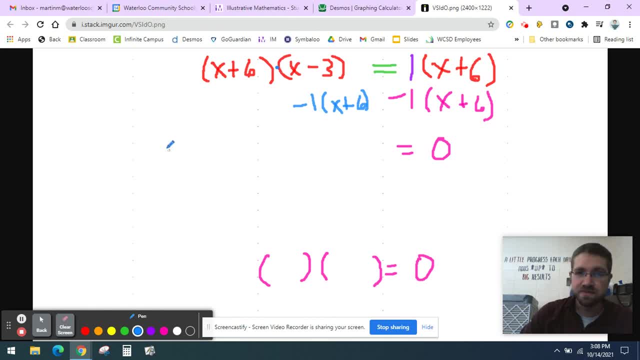 I can't take that away. okay. What I can do is write the two terms out side by side. It's going to look funny, but I'm going to do it anyway. Here I go: x plus six times, x minus three. 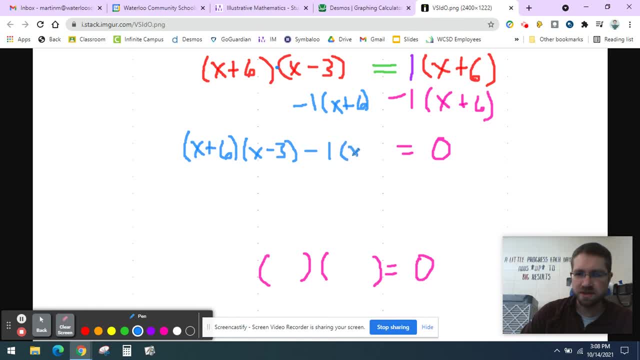 And then I'll have the minus one times x plus six over here. Now, having accomplished that, here's where it gets extra wacky. So what I notice is that both of these terms- and when I say terms there's two of them here- right A term is, you know, when you've got stuff separated by a negative. 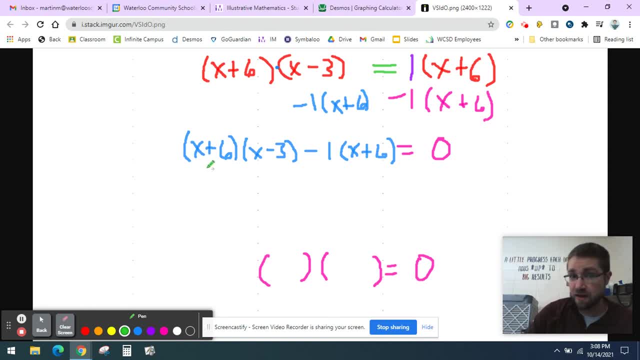 sign. okay, These two terms have a common factor of x plus six. They both have that. So what I'm going to do: if you have two numbers and they're both being multiplied by the same thing, you can factor it out, which is like taking that number and pulling it to the outside- Normally the outside. 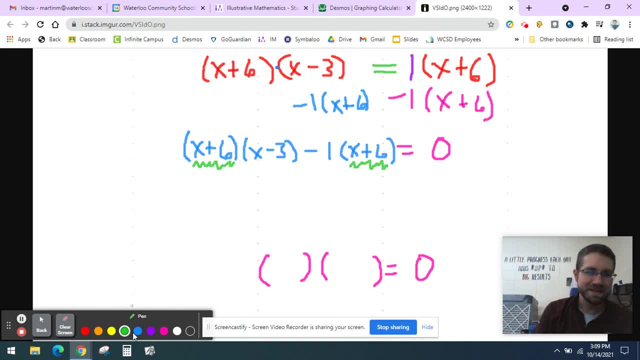 is over here Pulling it to the outside, you're finding away from both of those terms. okay, And so here's what that'll look like: I'll take x plus six and I'll put it on the outside here, And then I'll ask myself: well, if I divided x plus six? 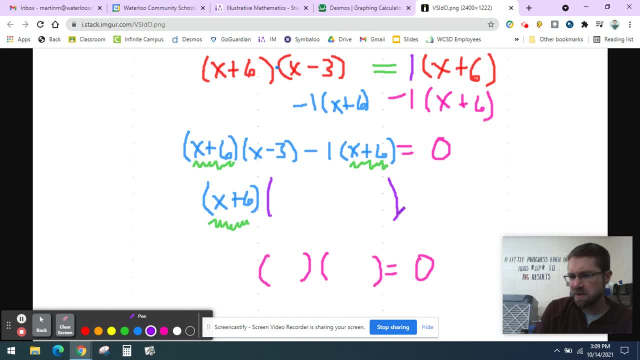 out of both of those things. well then, what would be left? What would be left from those two terms? Well, what's left over? Well, this still has the x minus three, And this would still have the negative one. So that's what's going to be left over, after I do. 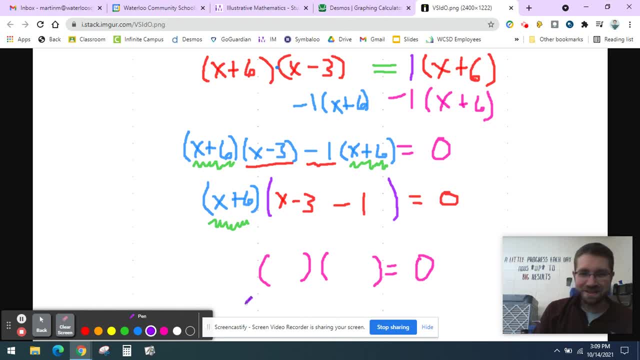 my factoring And this is really close to what I wanted, because I can see now that I've got x plus six in here And if I simplify what's inside of those parentheses, I would have x minus four, And this allows me to use the zero product property. I ask myself: okay? 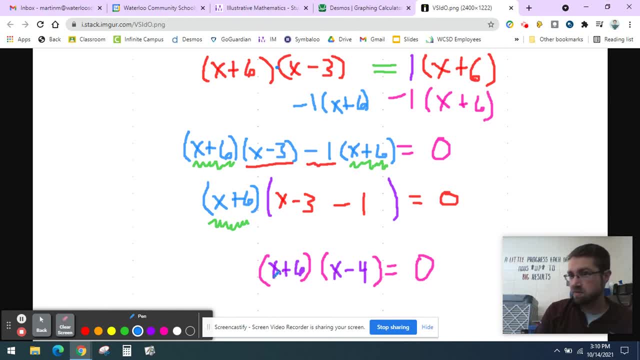 if two of these terms are equal to x plus six, what would be left? Well, if two of these terms are multiplied together equal to zero, what makes them equal zero? Well, obviously, if x equals negative six, then the first group will be equal to zero, And if x equals positive, 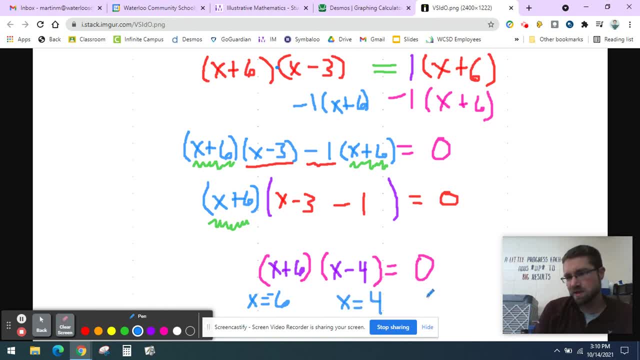 four, then the second group will be equal to zero. And those are my x values for my coordinate points, which we already knew. We already knew that they were going to intersect at four something and negative six something. Okay, But I'm finding intersection points, which implies that I have a y value as well. 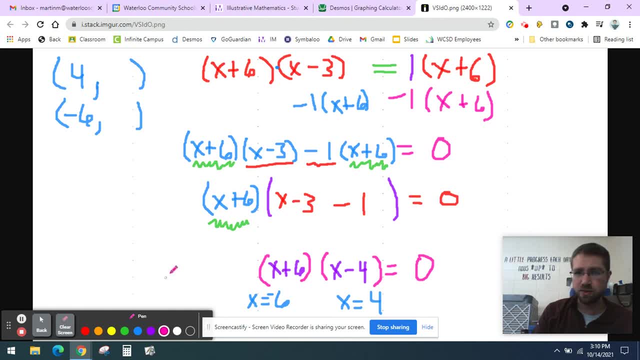 So now I need to go back and I need to find the y value for each of those equations. So if I was starting fresh, I would probably just choose the simpler equation x plus six and I would insert the numbers into that equation. Now, 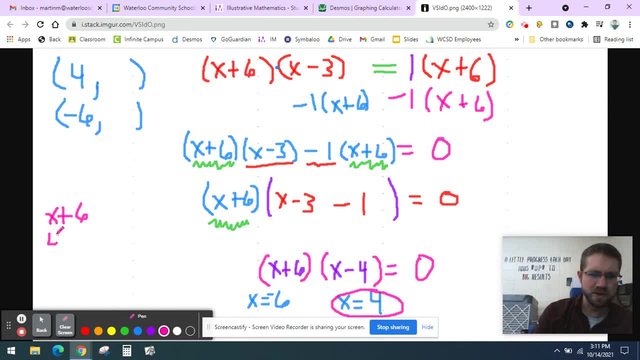 you already saw me do this at the beginning, if you watched the beginning. But if I replace x with four, I get ten, And we saw at the beginning that whichever equation you choose, you should get the same output. if these are the intersection points, Okay, And the other one was zero, So yeah, there's an example And that might be cool. 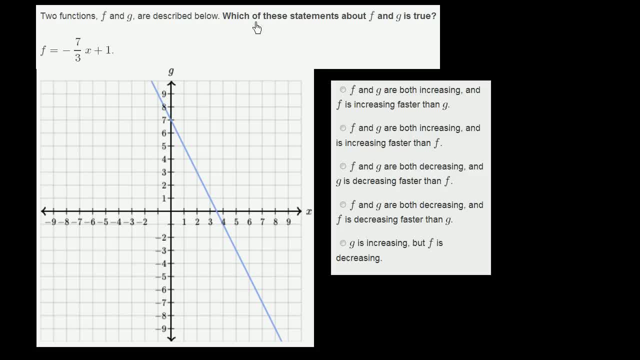 Two functions, f and g, are described below. Which of these statements about f and g is true? So they defined f as kind of a traditional linear equation right over here And this right over here is g. So this right over here is g of x. 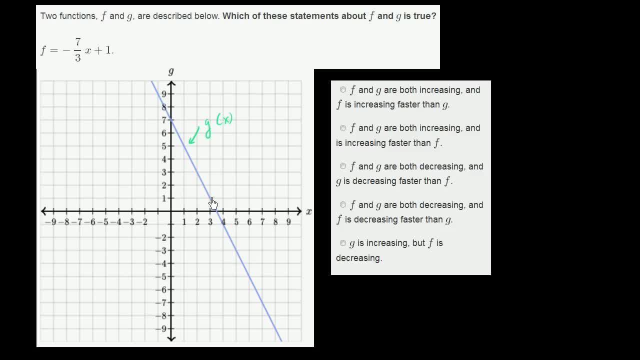 And that also looks like a linear function. We see it's kind of a downward sloping line. So let's look at our choices and see which of these are true. f and g are both increasing, And f is increasing faster than g. 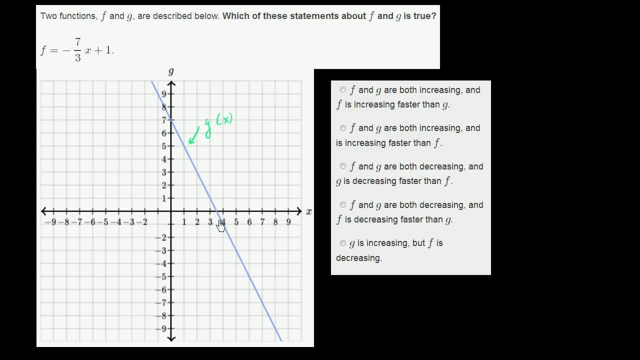 Well, when I look at g, well, first of all, g is definitely decreasing, So we already know that that's false. And f is also decreasing. We see here, it has a negative slope Every time we move forward. 3 in the x direction. 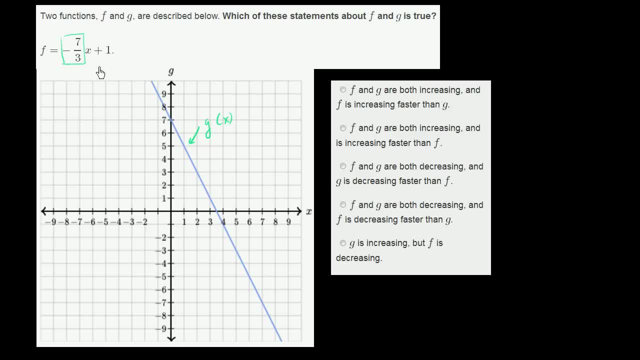 we're going to move down 7 in the vertical direction. So neither of these are increasing. So that's definitely not right. f and g are both increasing. Well, that's definitely not right. So we know that both f and g are decreasing. 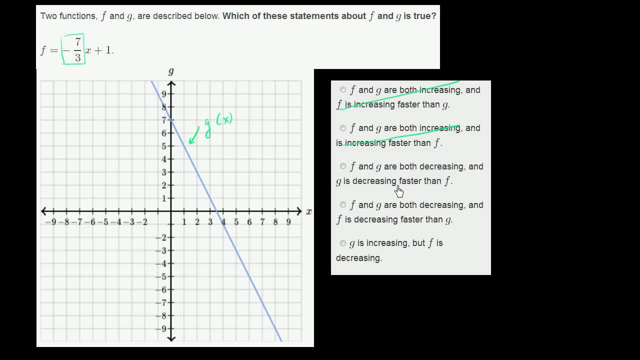 So this first choice is: they're both decreasing And g is decreasing faster than f. So let's see what the slope on g is. So the slope on g is, every time we move 1 in the x direction, positive 1 in the x direction. 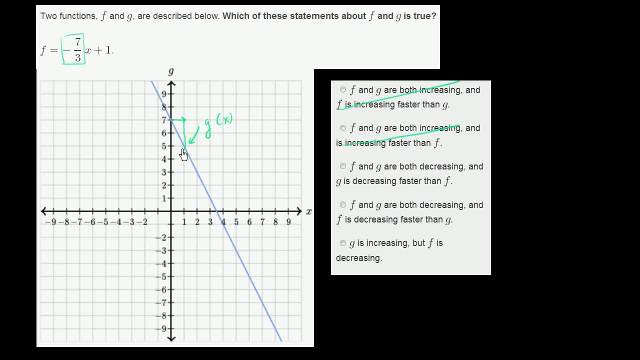 we move down 2 in the y direction. So for g of x, if we were to write our change in y over our change in x, Which is our slope, Our change in y over our change in x, When we move 1 in the x direction.